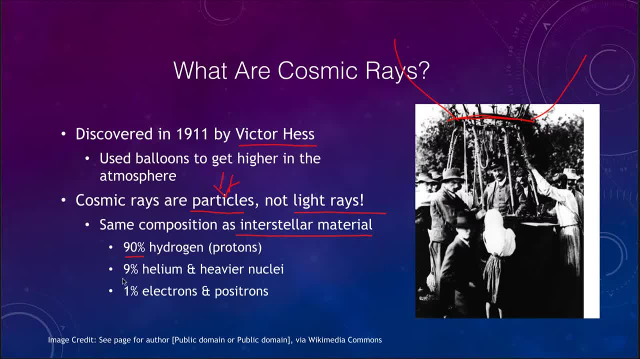 They are about 90% hydrogen, nuclei, protons, About 9% helium or heavier nuclei And about 1% are electrons and positrons and, if you recall, the positron is the antiparticle of the electron, So it is an antiparticle of the electron. 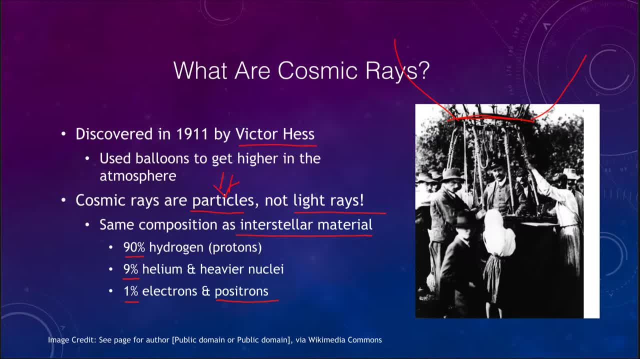 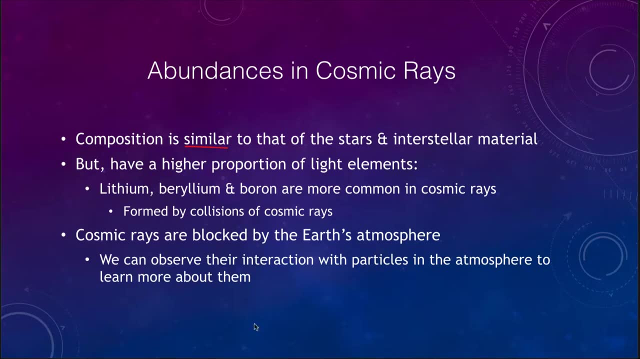 Now, when we look at these, there are some differences that we see. So overall, the rough composition is similar, but there are some differences compared to other things that we've seen, And when we look at the abundances of things in cosmic rays, we said that they're similar. 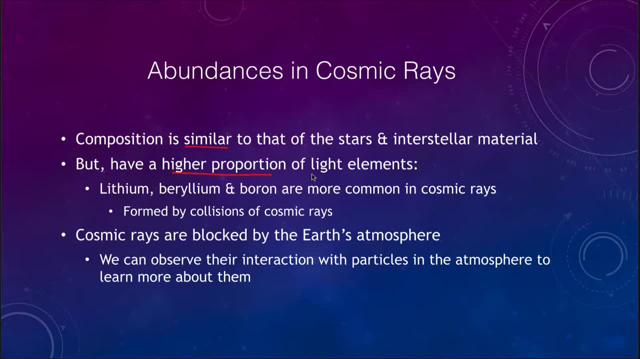 to them, but they have a higher proportion of the light elements. So not heavier elements but the lighter elements And not light as in hydrogen and helium. Hydrogen and helium make up the vast majority of everything that we see, But the three elements in the periodic 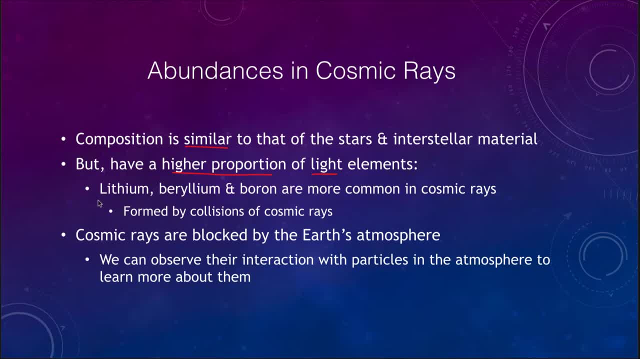 table that come after hydrogen and helium are the same And they don't have a different hydrogen and helium that are relatively rare. Lithium, beryllium and boron are very rare elements in the universe and what happens is when we form helium. 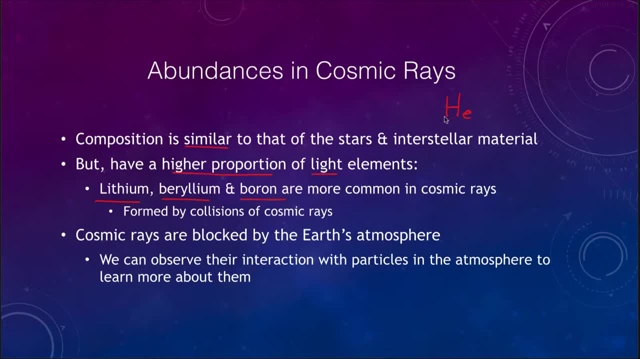 helium fusion in stars you have three helium atoms fusing to form one carbon atom. So three helium atoms combined together and we jump over these elements. and that's because if we try to use two helium atoms together, the product is unstable and immediately breaks apart. So the only way to form heavier elements in 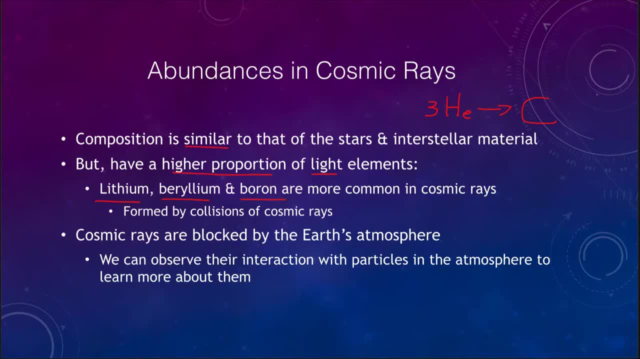 stars is to skip over these. So where do they come from? Well, we believe that they are formed by these cosmic rays and collisions within cosmic rays. So much of the lithium, beryllium and boron that we see is formed not in stars, as ever other. 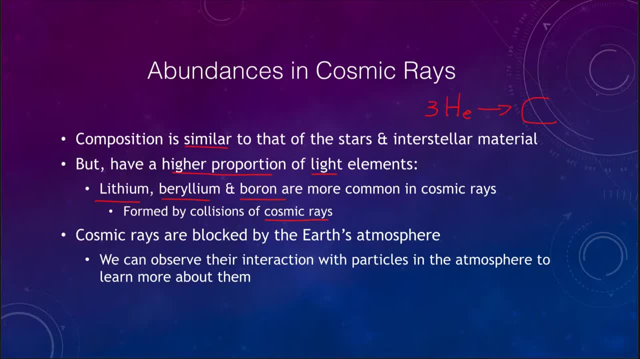 elements are, but is actually formed in cosmic rays. and that's because, if we try to fuse two helium atoms together, the product is these high-energy particles streaming through the universe and occasionally colliding with each other, and those helium nuclei and those protons could then form these slightly heavier elements. Now, fortunately for us, as I've 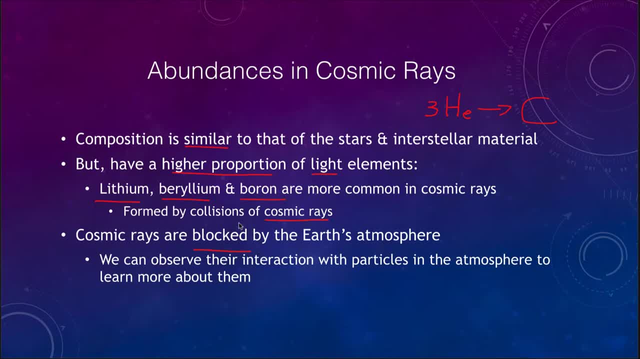 mentioned, cosmic rays are blocked by the atmosphere of the earth, so they are unable to get through the Earth's atmosphere. How do we detect them from the surface of the earth? Well, that's hard, but there are ways to do it. We can observe their interaction with particles in the atmosphere. So when they 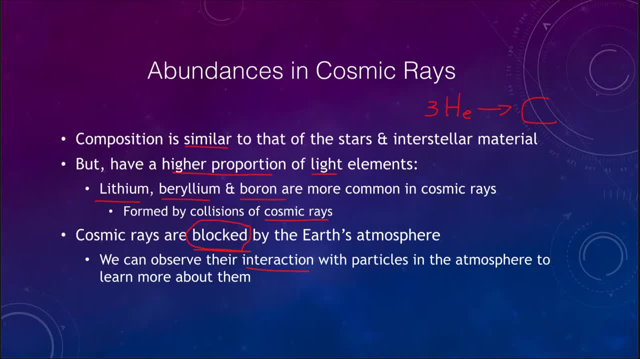 collide in the upper atmosphere, they produce a stream of high-energy particles and we can use those to work backwards and figure out something about the cosmic rays. So we take these interactions, use them to learn more about the cosmic rays itself, even though from the earth's surface we cannot see. 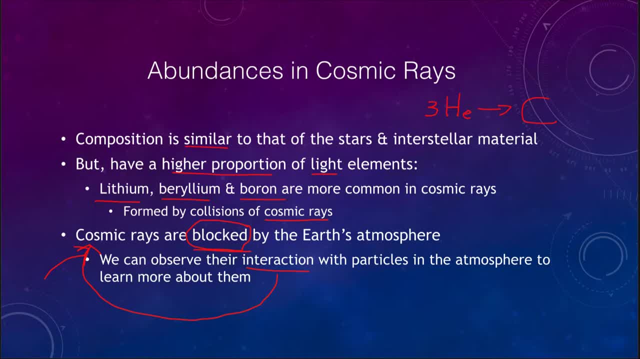 them directly. Now, other ways would, of course, be to get up to the surface of the earth- If you're up above the Earth's atmosphere- to observe these. If you're up above the Earth's atmosphere, then you would be able to detect the cosmic rays directly. 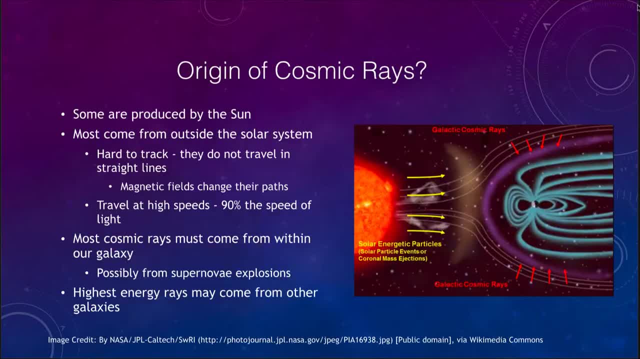 Now, where do these come from? Some of these cosmic rays are produced by the Sun, but the vast majority come from outside of the solar system. They are not a part of our solar system, and the difficulty with them, as compared to light rays, is that they are very hard to track. They do not travel. 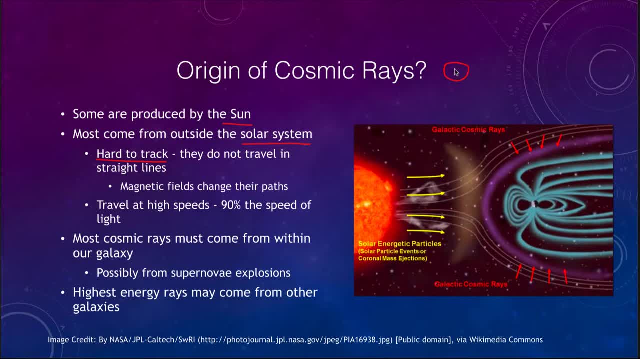 in straight lines. So if we have a source over here of the particles and we're over here on the earth, light, electromagnetic radiation will travel in straight lines pretty much and come to us right here on earth. However, these other ones can travel and will travel along the magnetic field. so 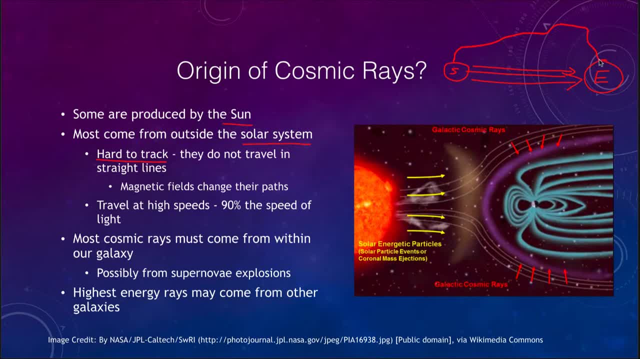 they can follow long winding paths to get to us here on earth and therefore, how do we know where they came from from? When it comes from this direction, we see it as coming from out here, whereas the real source was over here. So magnetic fields can change these paths. 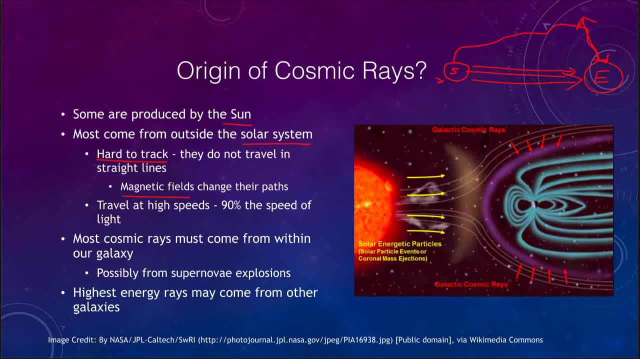 of particles that they cannot do to electromagnetic radiation. They do travel at high speeds. they travel at about 90% of the speed of light, so a little bit slower than the light and the electromagnetic radiation itself, but they do travel still at very, very high speeds. Most of them come from outside. 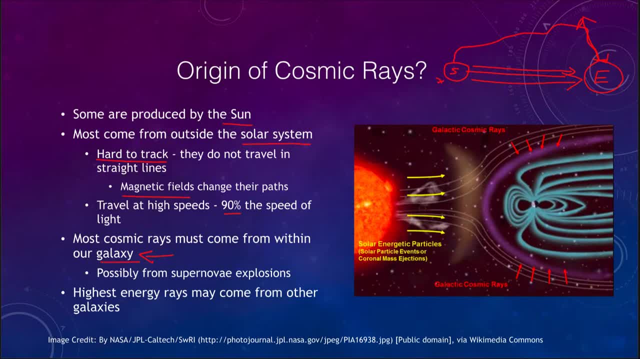 our solar system and they do come from within our galaxy. We think that perhaps supernova explosions cause give us a lot of these cosmic rays and that would be in a massive explosion, would send out streams of these particles that could eventually just travel. it would be traveling through space and remember as 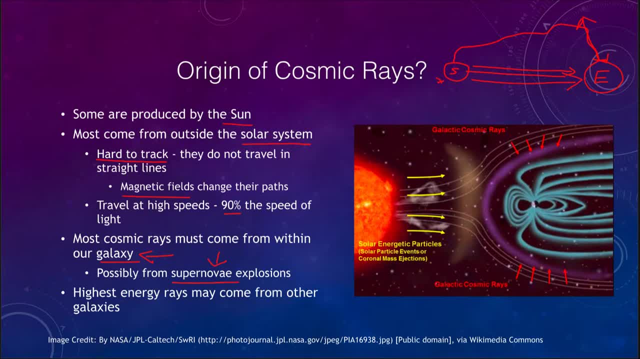 they travel through space. there is nothing to slow them down, They just keep traveling. so if they are emitted at very high energies, they continue to move at those very high energies. So they could travel there for thousands or millions of years at those very high speeds until they eventually strike something like the Earth. But the very 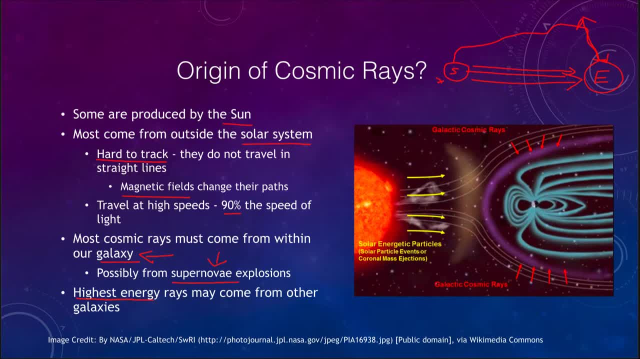 highest energy ones that we see could actually come from other galaxies. So they could come from outside our galaxy and stream here And stream into the Earth as well. So when we look at our image here, we do have some that are coming from the Sun, from perhaps a coronal mass ejection charged. 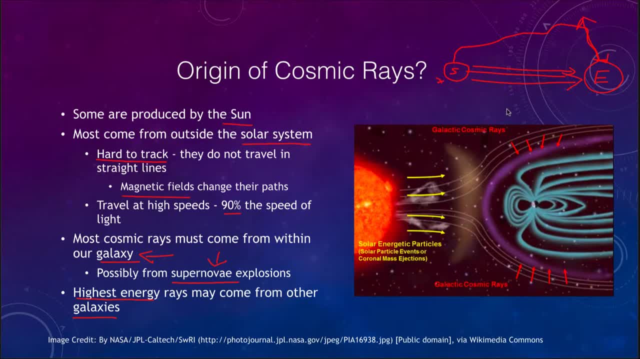 particles coming out, those would strike the Earth's magnetic field. There could be galactic cosmic rays coming from all other directions and there could be those very high ones that are actually coming from other galaxies and maybe even more energetic events. So how do we go about detecting these? 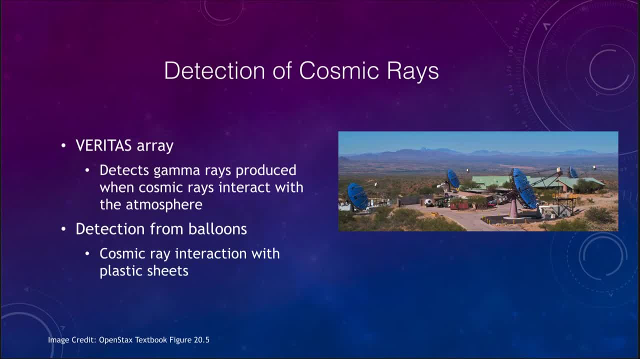 Well, there's a couple ways that we can do this. One is the Veritas Array, and that detects not the cosmic rays themselves. You can see the image here: it's actually on the surface of the Earth, so the cosmic rays are not going to make it. 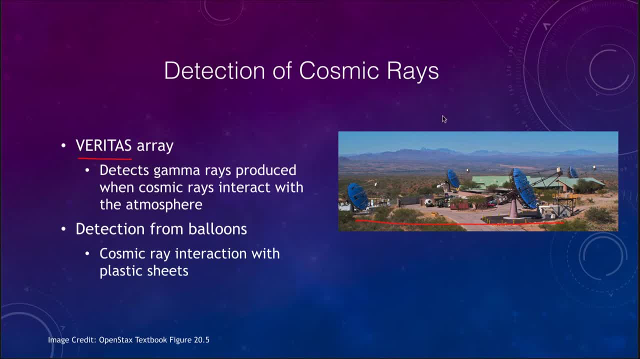 down to the surface of the Earth. But when those cosmic rays strike particles in the Earth's atmosphere, so they strike a particle here that will then produce gamma rays which can then come down to the Earth and be detected. So the particle itself does not make it to the Earth. this is the particle, but it 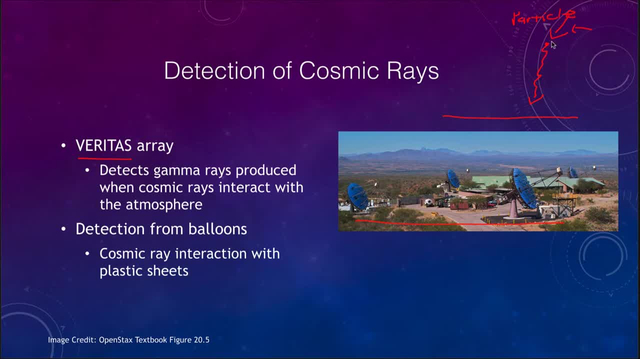 does not make it to the surface of the Earth. However, other gamma rays can be detected and these can detect those flashes of gamma radiation that come down to the Earth from these particles and can then trace back and learn. try to learn a little bit more about these cosmic rays. We can also use balloons.